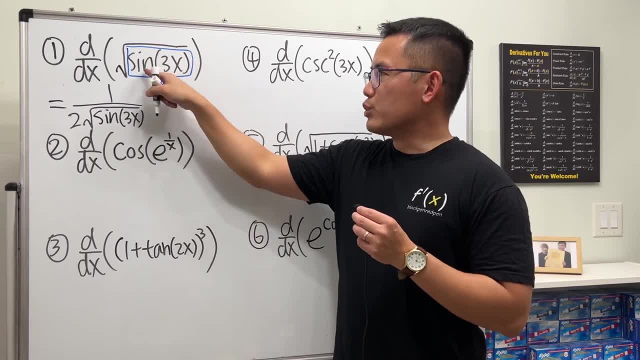 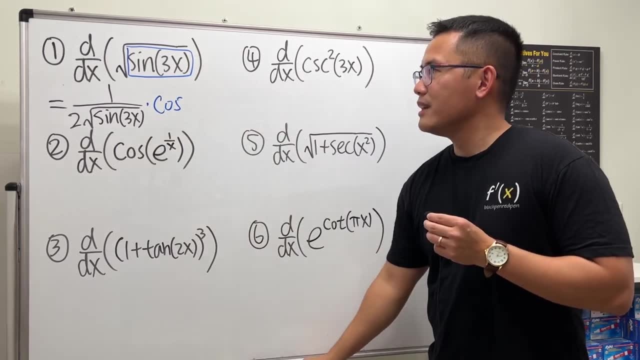 Then we are going to differentiate the inside: The derivative of sine is cosine of 3x. And then we are going to differentiate the inside: The derivative of sine is cosine. So we multiply by cosine, But as you can see here, inside we have the 3x. 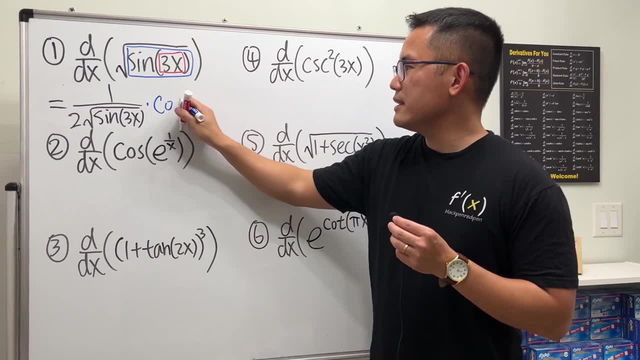 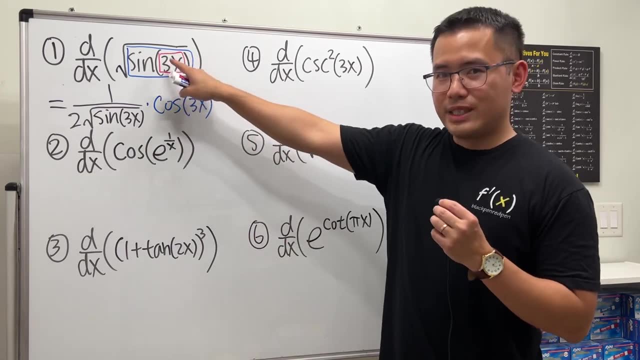 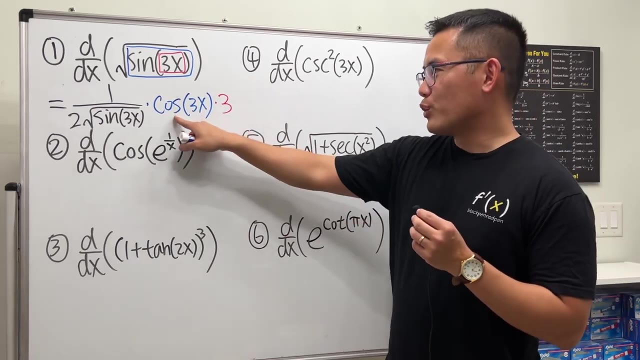 So the 3x stays inside of the cosine. And then the last step is we have to look what's inside the box. The derivative for the 3x is 3.. So multiply by 3.. That's it. So the chain rule one time. and then here's the chain rule for the. 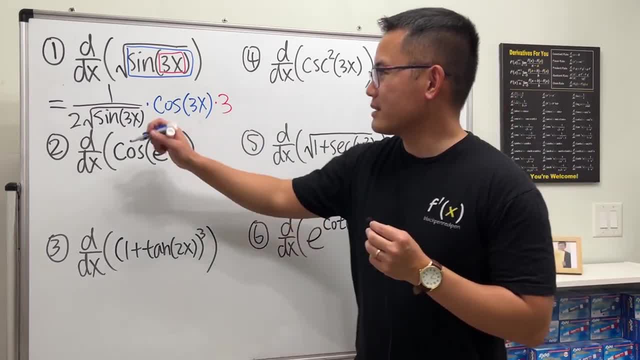 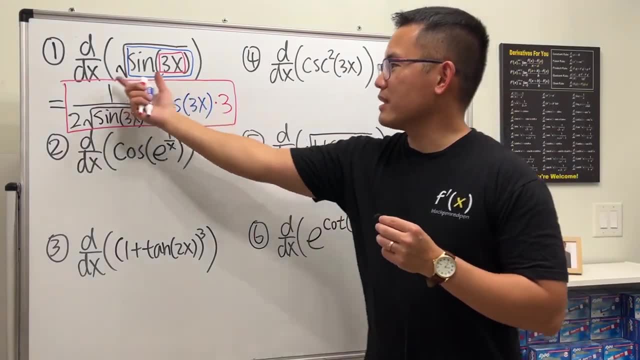 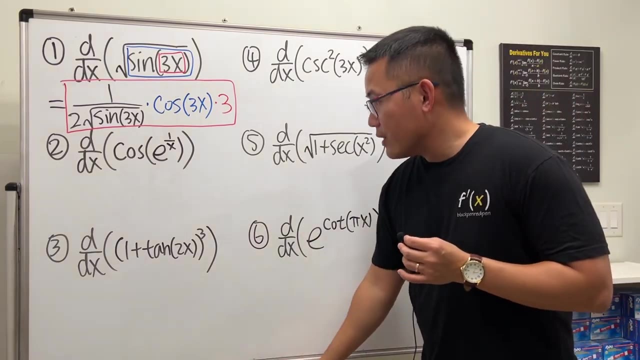 second time. So that's it. Oh, the box is in red to make it stand out more. And I'm not going to simplify. You can put this on top and all that, But let's just focus on the derivative, the calculus steps, all right. All right for the number two. here we have. 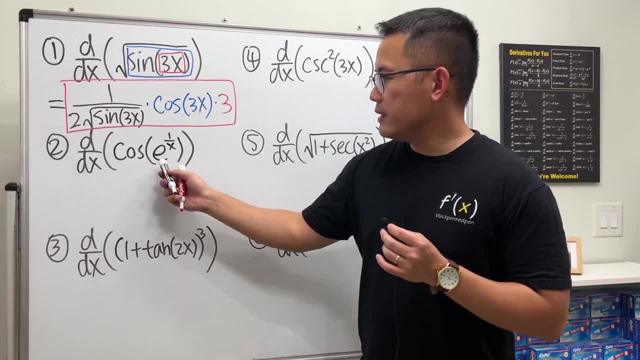 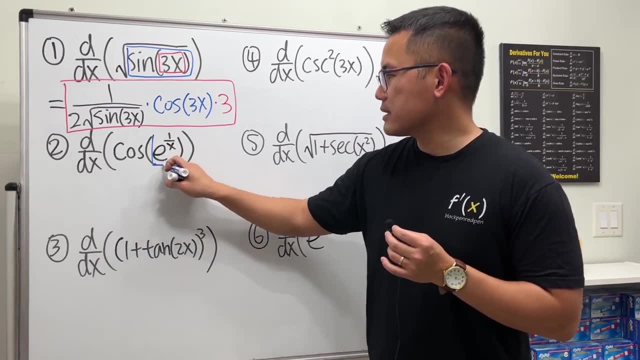 the derivative for cosine of e to the 1 over x. So, as you can see, the outer function is the cosine. So we have cosine of the box. What's the derivative for cosine of e to the 1 over x? What's the derivative for cosine of e to the 1 over x? What's the derivative for cosine of e to the 1 over x? 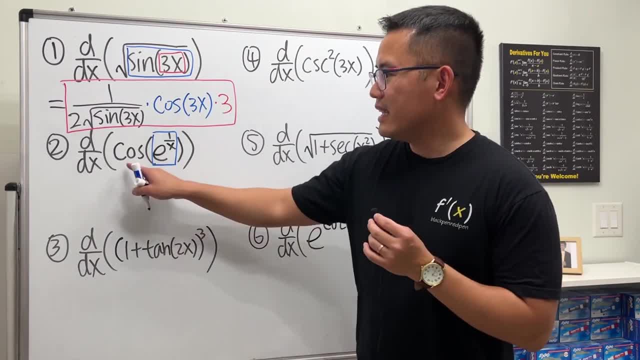 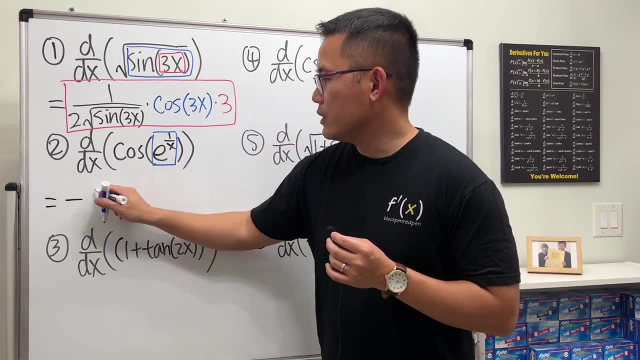 We have the derivative for sine of x. What's the derivative for cosine of e to the 1 over x? So we have the derivative for sine and cosine of best friends right, And the derivative of the co-function is negative. So we will first get negative and then we get sine, because sine and 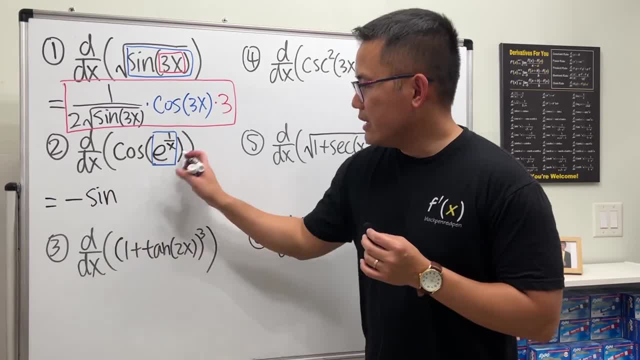 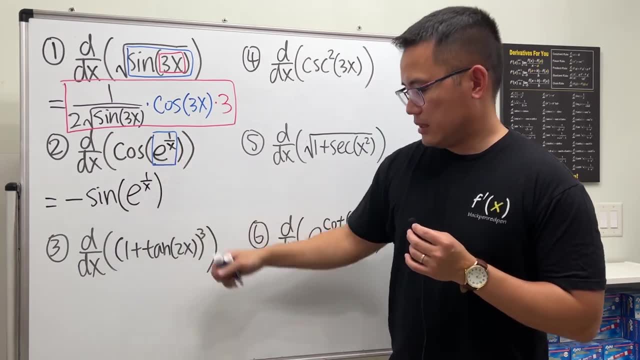 cosine are best friends in calculus. And then the inside stays with right down e to the 1 over x, And then we differentiate this and the derivative of e to the 1 over x And the 1 over x is really like another function. 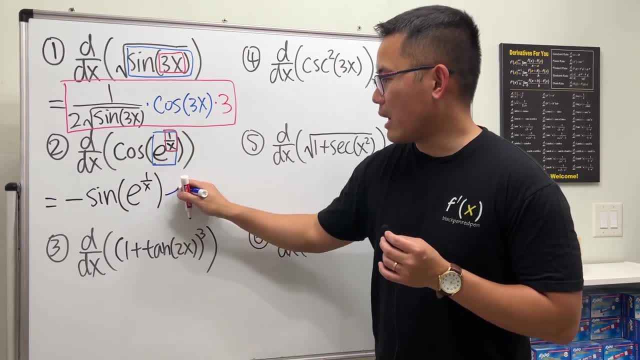 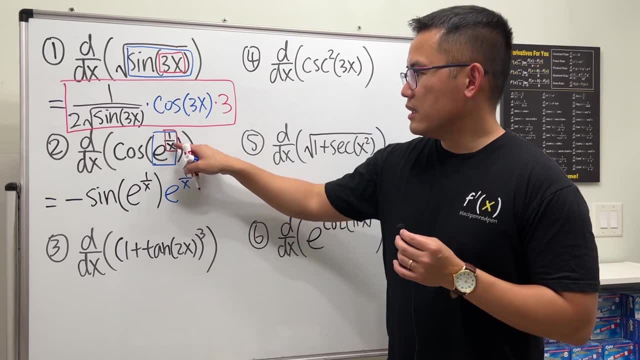 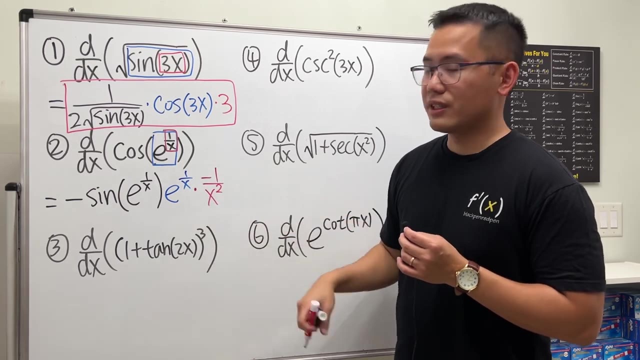 The derivative of e to the box is e to the box, which is just that. again, Just repeat that. But finally we differentiate the very inside, the derivative of 1 over x, which is negative: 1 over x, squared, Just like that. 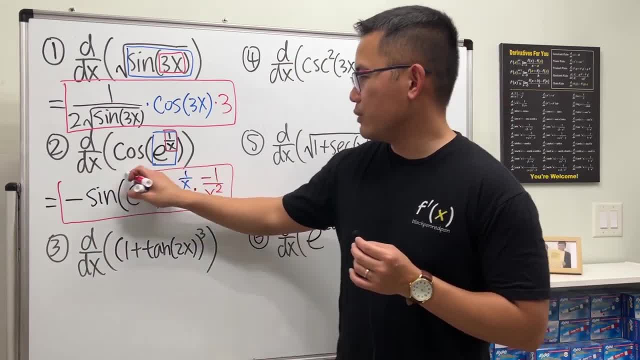 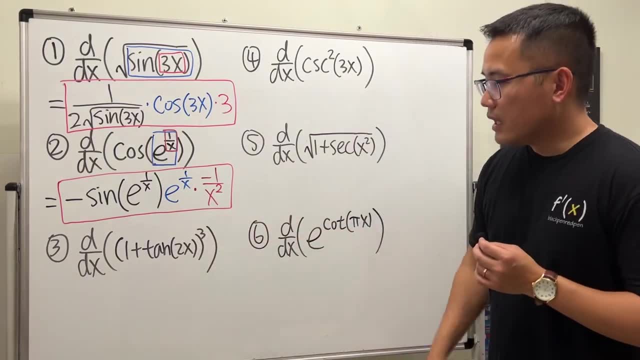 And again we are done. Negative times. a negative is positive, but I will leave that to you guys. I think this is more clear on what exactly to get the derivative. Now number 3.. As we can see, the outer function is this: to the third power: 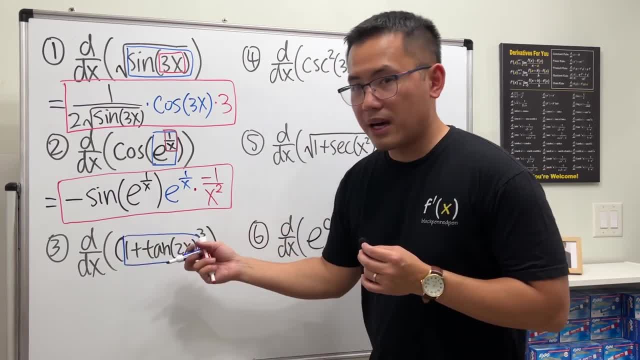 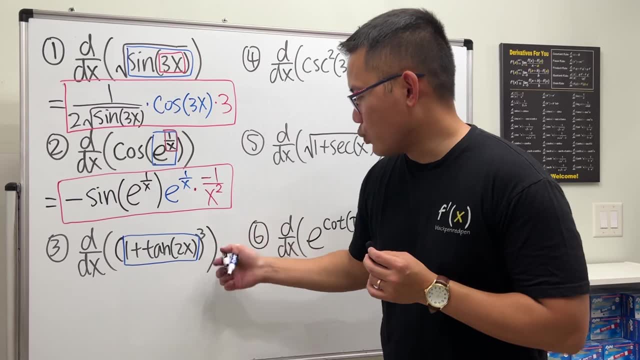 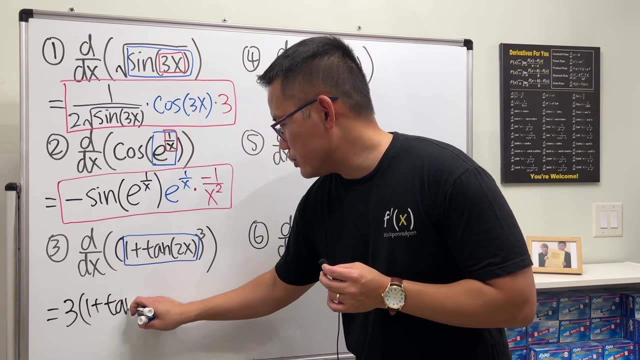 So we really have this thing as like the box to the third power. That said, we will have to use the power rule. first, Bring the 3 to the front and minus 1.. So the first step is we have 3, and then inside is 1 plus tangent and then the 2x. 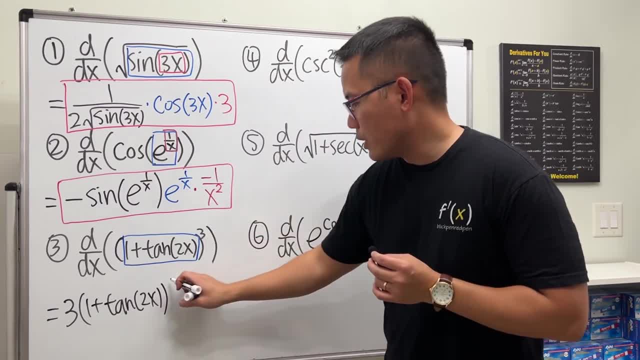 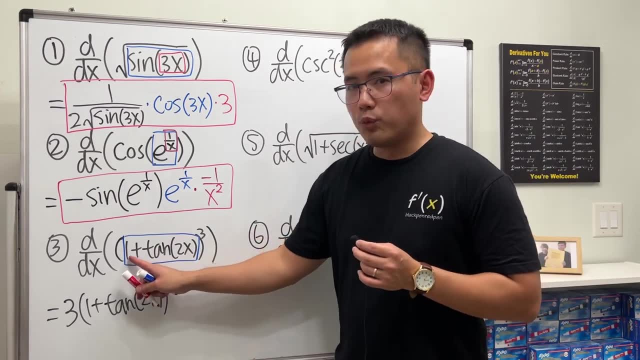 Just write that down. And 3 minus 1, we get the second. All right, now we are going to differentiate the inside. The derivative of 1 is just 0.. The derivative of tangent: Tangent and secant are best friends in calculus. 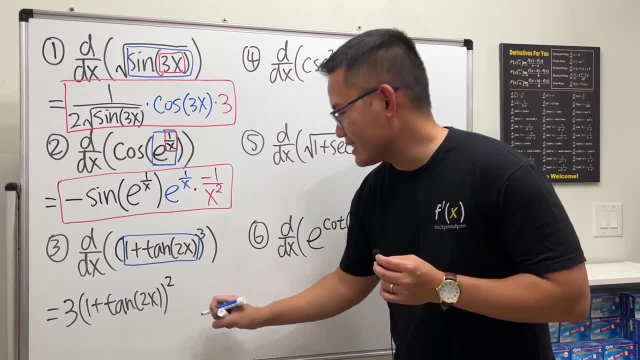 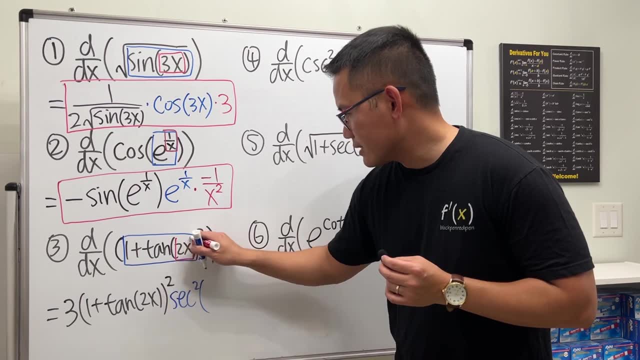 The derivative of tangent is secant, but to the second power. You have to remember that. So we multiply by secant to the second power, and then we also have that inside, which is the 2x. So maintain that 2x. 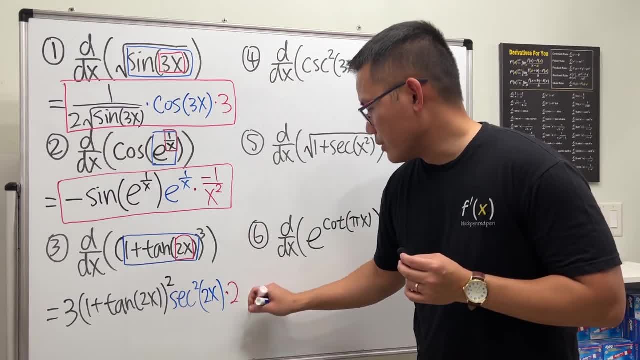 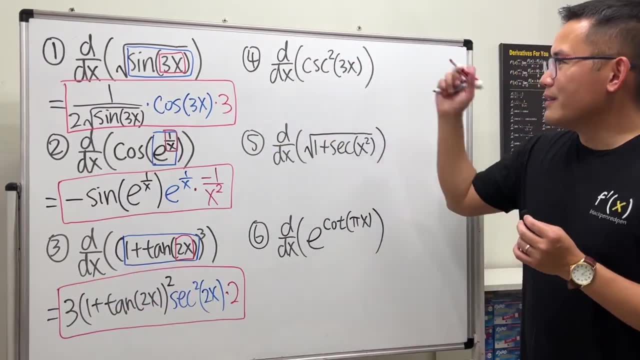 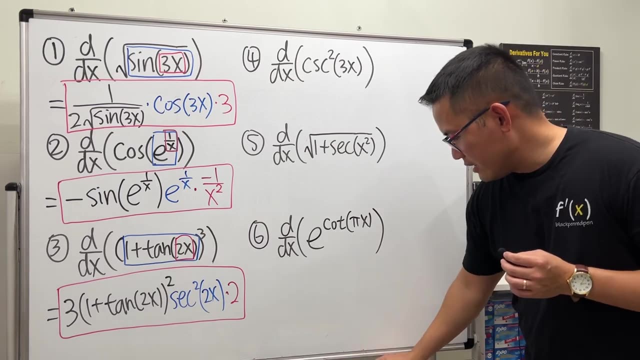 Take the derivative of 2x, which is 2. So Multiply by that, That's it Now, number 4.. We have cosecant square of 3x And this notation. it's really like saying the following: 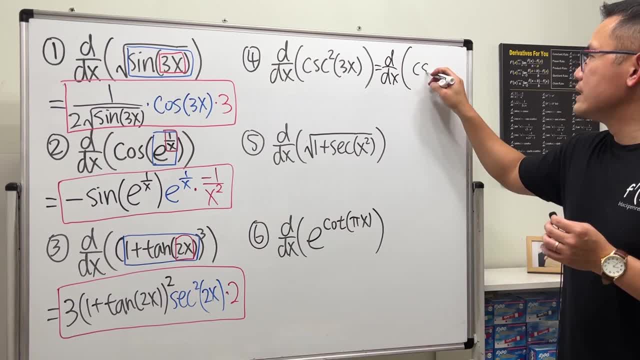 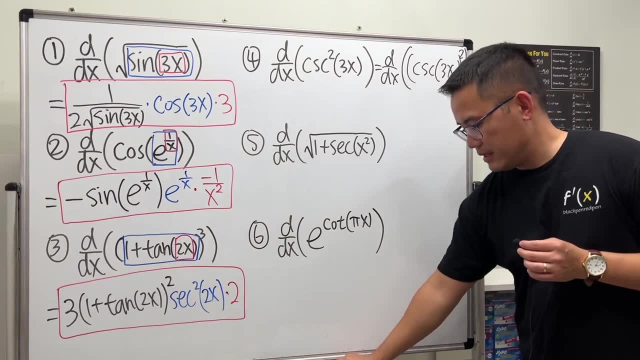 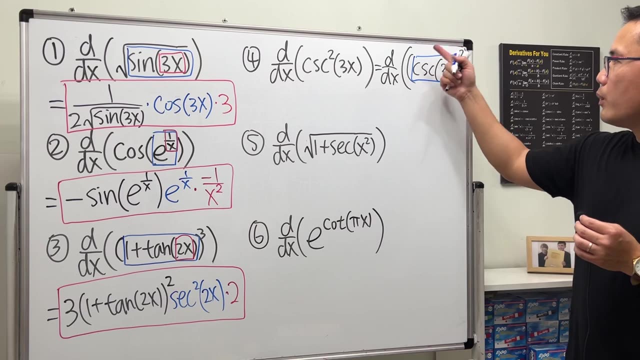 This is the same as saying taking the derivative of cosecant 3x and then square. So what we really have is an input like a box, like this, And then to the second power. So bring the power to the front and minus 1.. 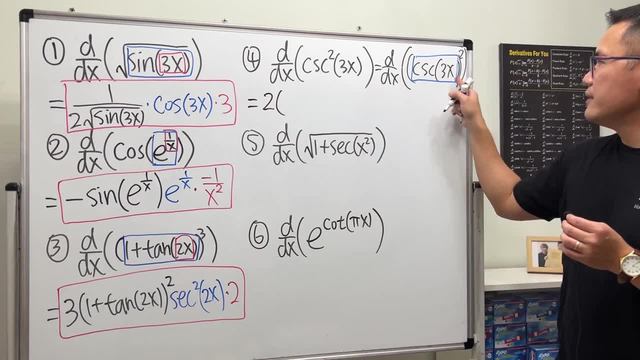 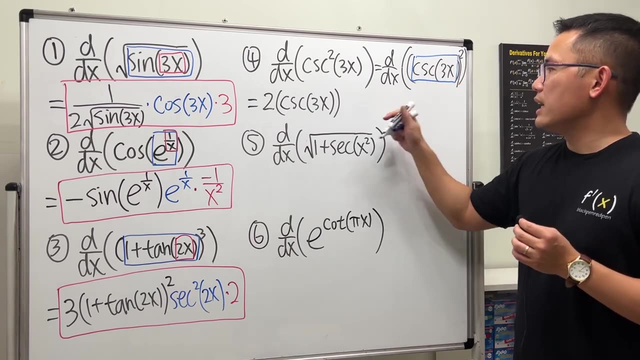 So first we will have 2 at the front and then the in the function for the box right. So cosecant of 3x to the first power, because 2 minus 1.. Then we differentiate: the inside Derivative of cosecant is negative cosecant also with cotangent. 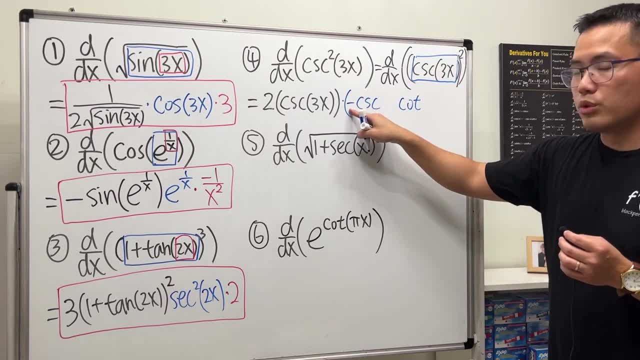 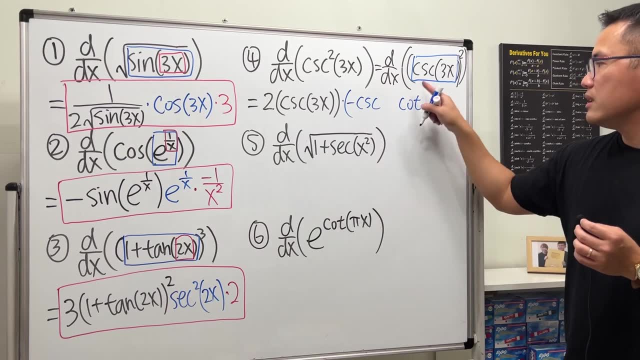 First, remember co-function. we have negative derivative, and cosecant and cotangent are best friends. Cosecant is the one that repeats, just like secant, And you also can find its best friend here, which is cotangent. And then the input, which is 3x. 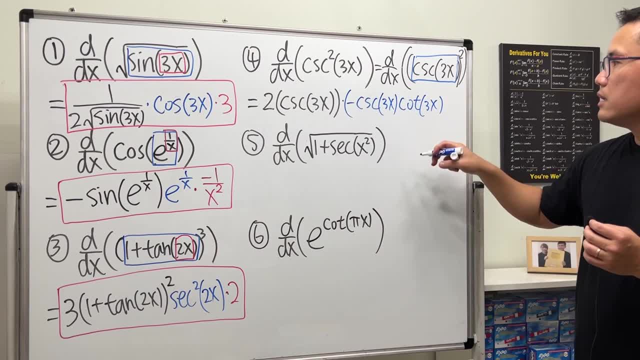 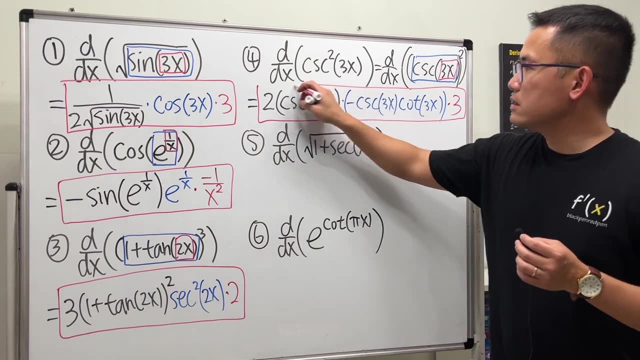 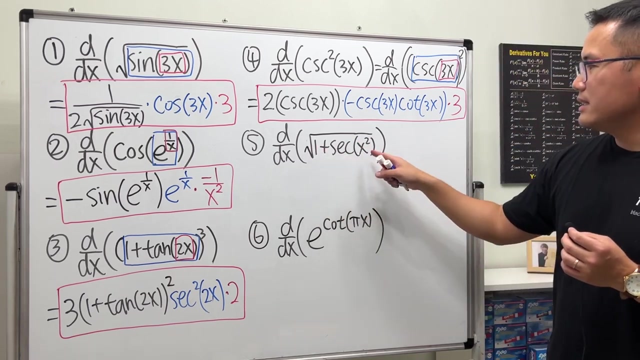 Just maintain that. So that's that part. And finally notice that the very inside the 3x, the derivative of that is 3.. So just like that. So this right here is the derivative of that. Next, we have square root of 1 plus secant x, squared. 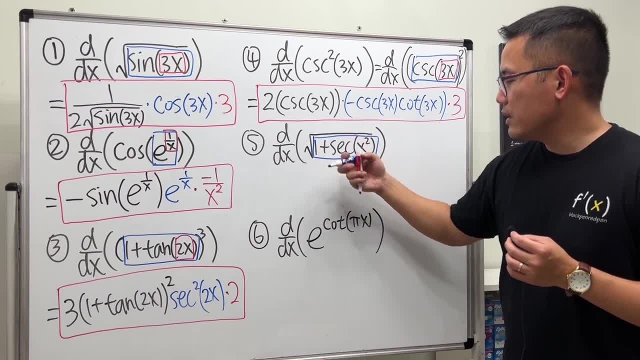 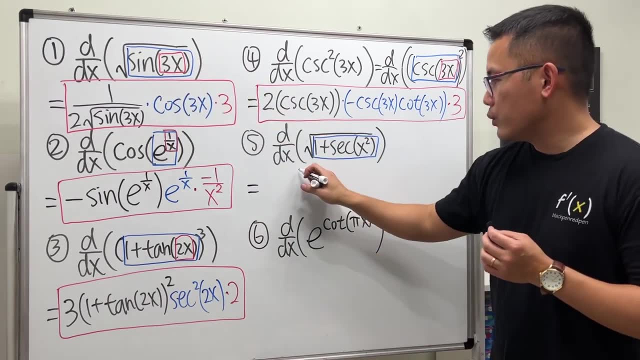 So we can see that this right here is the in the function. Therefore, we are going to first differentiate the square root. So that's that for that We have 1 over 2 square root, Just put inside here 1 plus. 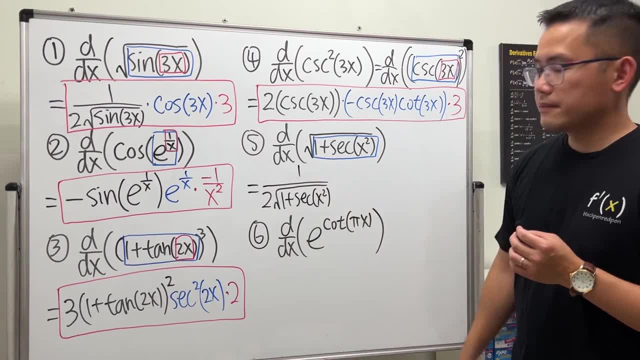 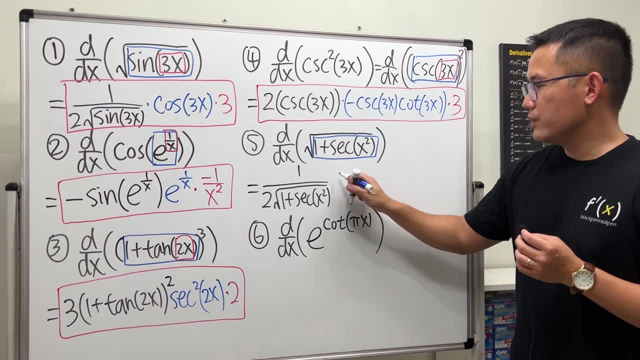 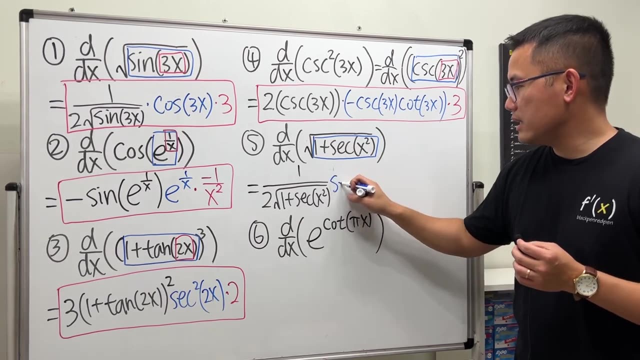 secant of x squared. And then we differentiate inside: Derivative of 1 is 0.. Derivative of secant. Well, yes, It's going to be secant and tangent. So let's write down secant And remember. you just maintain inside: 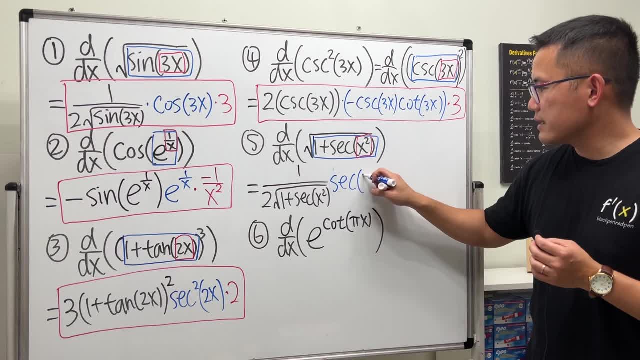 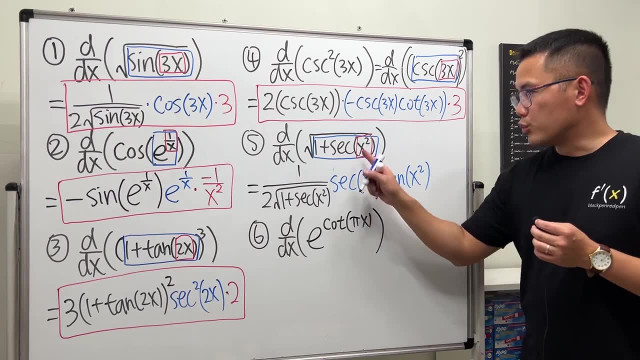 This is like a box right here, right. So secant of x- squared, And also we need a tangent, And also we need a tangent Of x squared, Derivative of secant. Firstly repeat, And then you also invite its best friend, which is tangent. 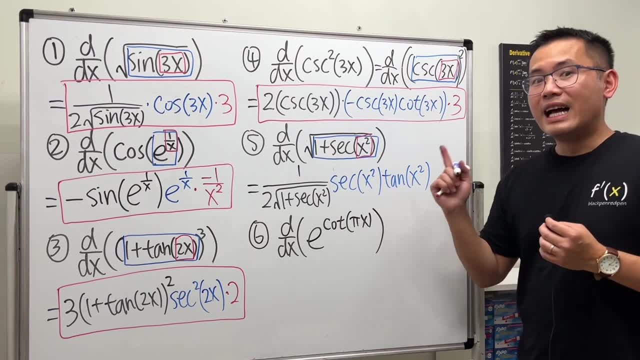 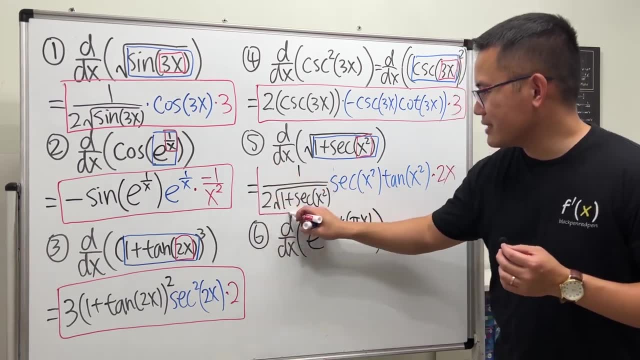 And you just maintain the x squared inside for both of them. Lastly, the derivative of x squared is 2x, So we multiply by 2x, Just like that. So chain rule twice. I will tell you it's not so bad. 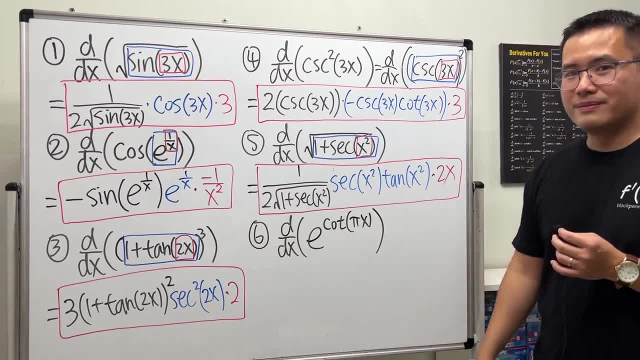 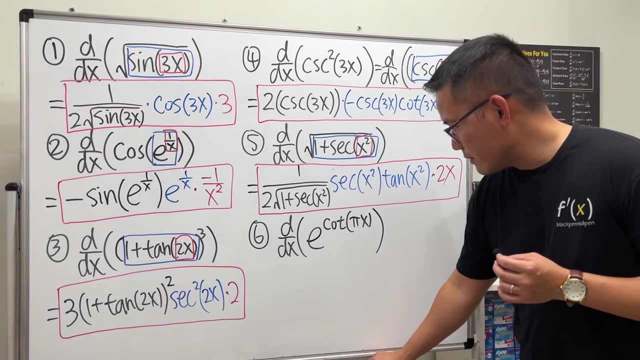 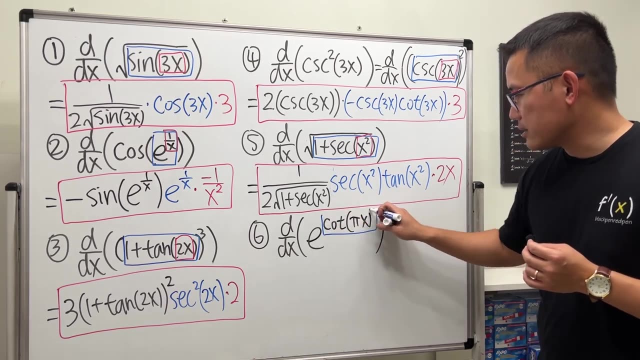 Just kind of calm down Practice a few more. You should just try the last one before you watch this douche. Done, All right, Let's have a look First. here we have e to the cotangent, all that right. So it's e to the box, like so. 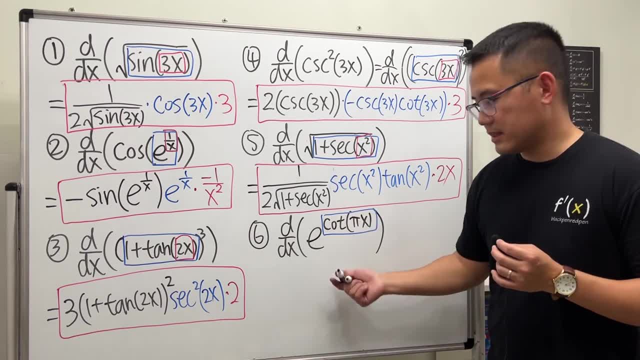 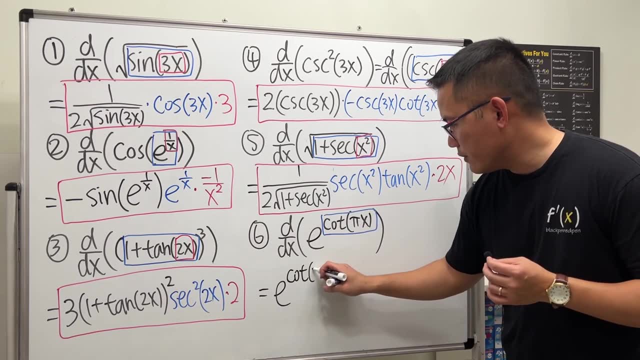 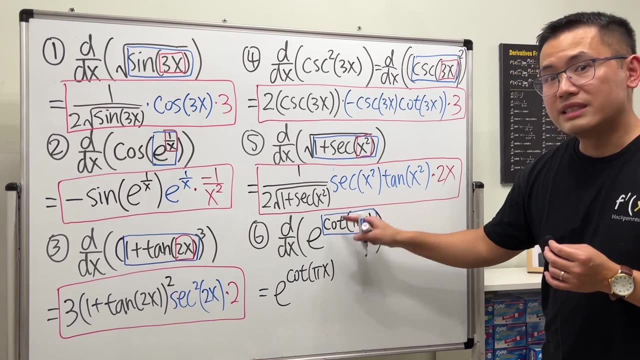 And the derivative of e to the box is just e to the box. So the first step is e And then we just repeat that in the exponent, So cotangent of pi- x. Then we differentiate the box. The derivative of cotangent is what co-function is: negative derivative.